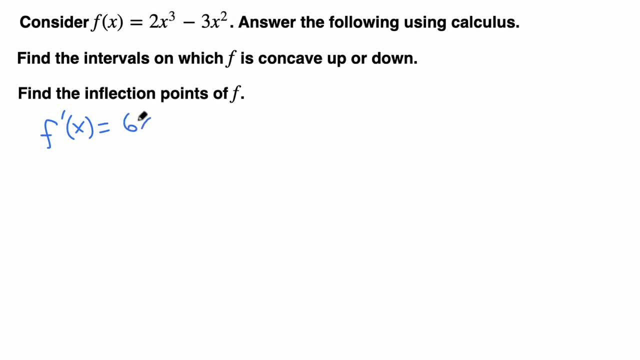 Derivative is 6x squared minus 6x, and second derivative is now 12x minus 6.. Okay, now we set the second derivative, 0, that is, 12x minus 6 equals 0. Isolate x, add 6 to the both sides and divide by. 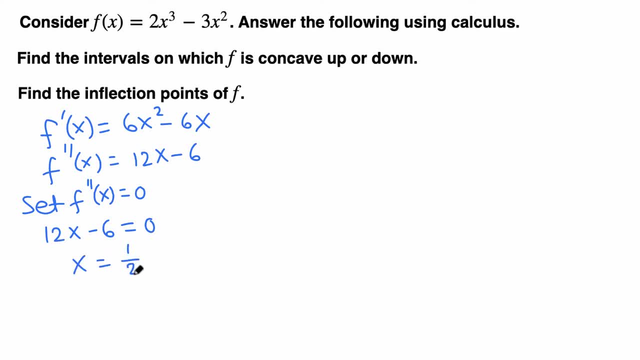 12.. So 6 over 12, which is 1 half. Okay, now we need to do the interval test. This is a polynomial, so it's defined everywhere- negative infinity through positive infinity- and we got a possible inflection point x-coordinate of inflection point 1, half somewhere, 1 half here. Now we pick a representative. 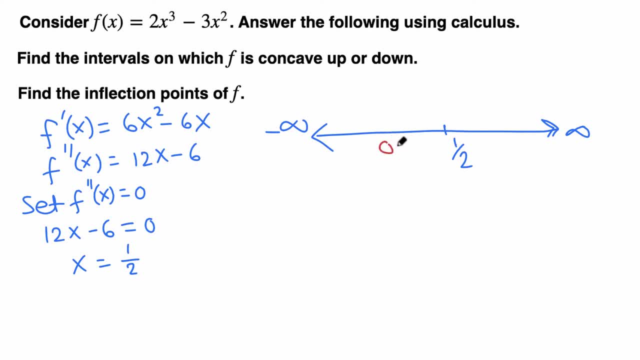 from each interval. you know, one half means we can pick 0, we can pick one and we plug this into second derivative. okay, which is here and see whether we get plus or minus. plug in zero here, zero second derivative. my bad, this is not second derivative, so we were supposed to plug in here second. 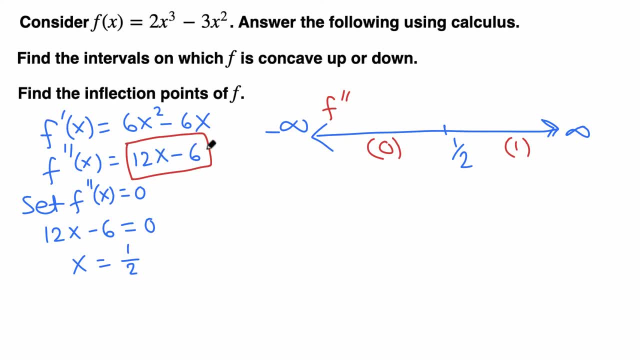 derivative. so plug in zero here to zero minus 6, negative. so we get second derivative negative and one plug in one here. 2 power minus 6 is positive. okay, and we know that when second derivative is negative then the function is concave downward and plus means concave upward. Now we can answer the first question. so 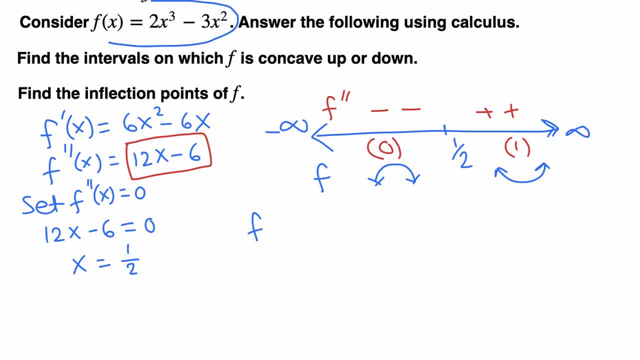 the function is positive. this given function, by the way, this given function is concave upward on here one half through positive infinity, concave downward, concave downward, or just concave down on here negative infinity through one half. okay, now to find the inflection points of F. look at here. we got one candidate, one half, and 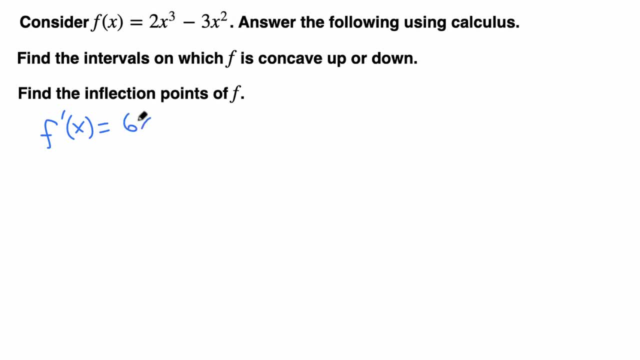 Derivative is 6x squared minus 6x, and second derivative is now 12x minus 6.. Okay, now we set the second derivative, 0, that is, 12x minus 6 equals 0. Isolate x, add 6 to the both sides and divide by. 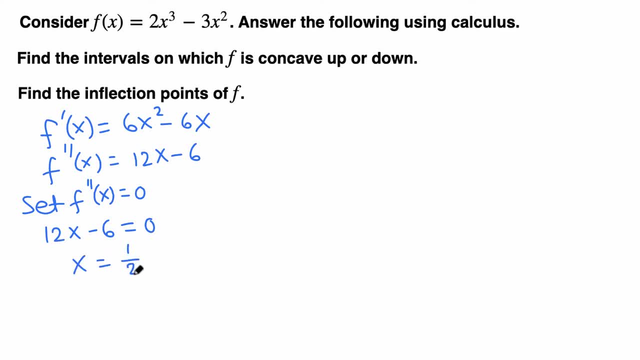 12.. So 6 over 12, which is 1 half. Okay, now we need to do the interval test. This is a polynomial, so it's defined everywhere- negative infinity through positive infinity- and we got a possible inflection point, the x coordinate of. 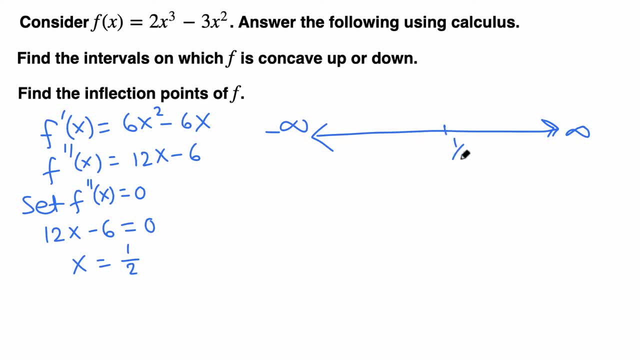 inflection point: 1, half somewhere, 1 half here. Now we pick a representative from each interval. you know, 1 half means we can pick 0, we can pick 1 and we plug this into second derivative okay, which is here, and see whether we get plus or minus. Plug in 0 here, 0 second derivative. my bad. 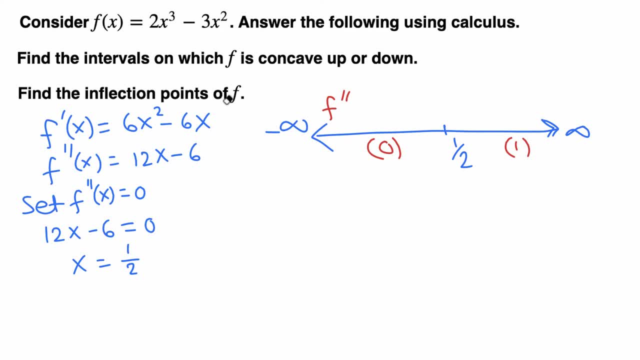 this is not second derivative, So we were supposed to plug in here second derivative. So plug in 0 here to 0 minus 0.. 0 minus 6 negative. so we get second derivative negative and 1. plug in 1 here. 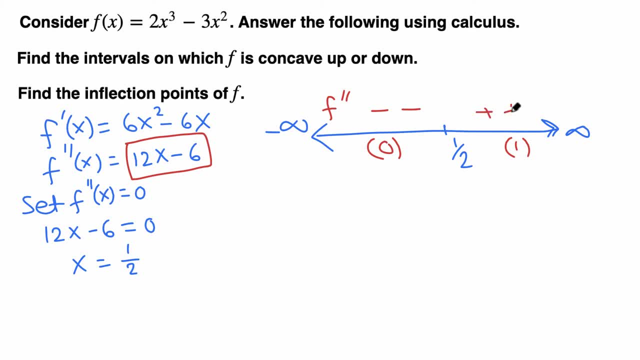 2, power minus 6 is positive, And we know that when second derivative is negative, then the function is concave downward And plus means concave upward. Now we can answer the first question. So the function, this given function, by the way. 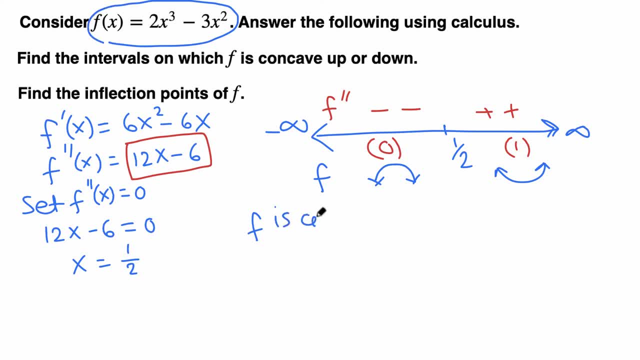 this given function is: concave upward on here one half through positive infinity, concave downward, concave downward or just concave down on here- negative infinity through one half. Okay, now to find the inflection points of F. look at here. we got one candidate, one half, and that's what. that was the case here, and